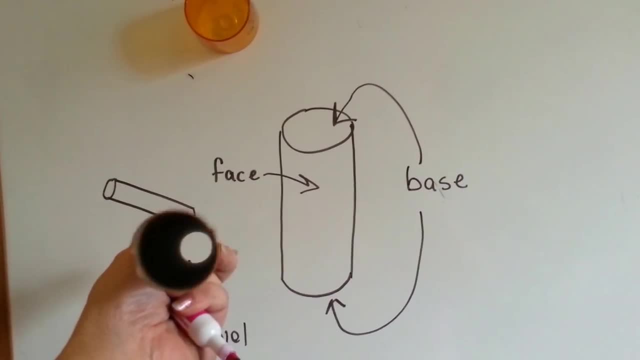 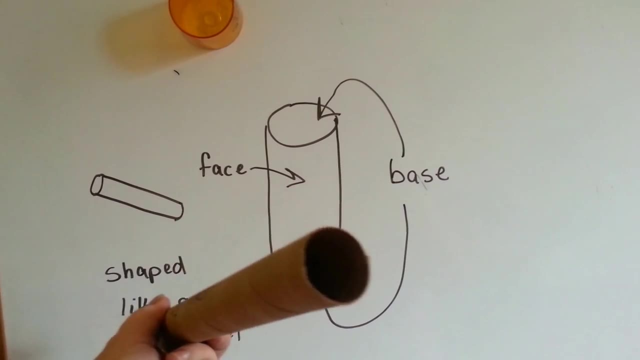 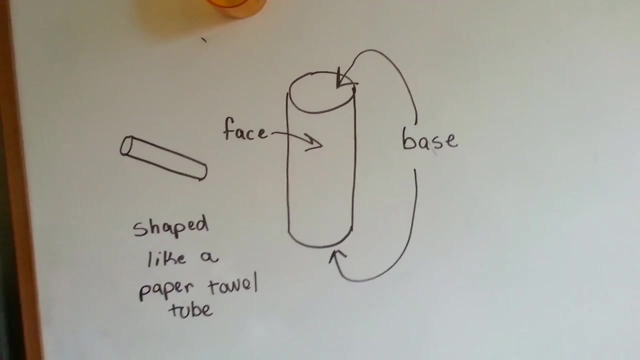 So this doesn't have the base on it because there's a hole, But you could tape ends to this and make bases, And you can still measure how big the hole is Where the base would be. Okay, The next shape I'm going to show you is the cone. 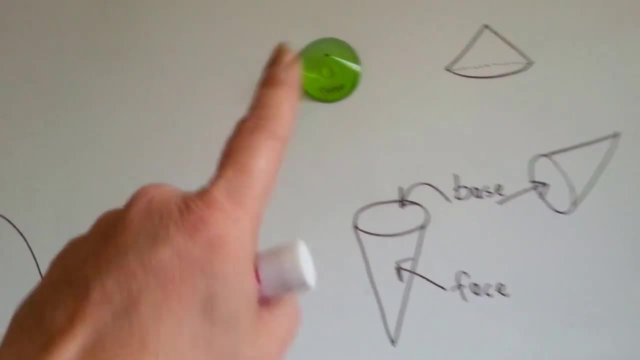 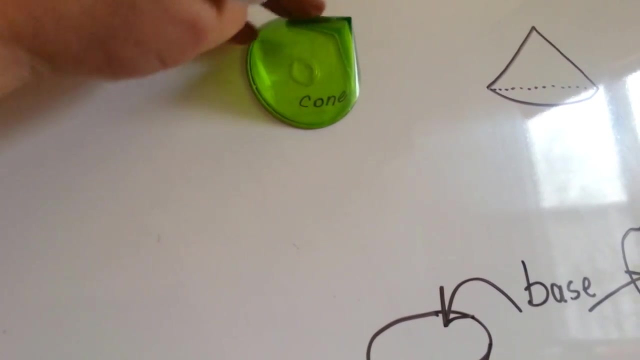 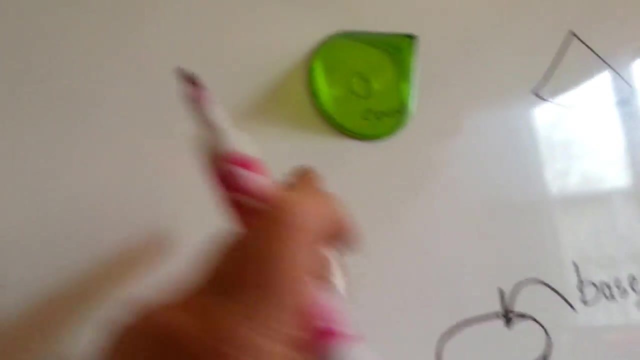 And it's just like an ice cream cone. See, Here's one on the board. This lateral face right here is where I wrote the word cone, And it's base, the round, flat, circular part, is stuck to the board See. 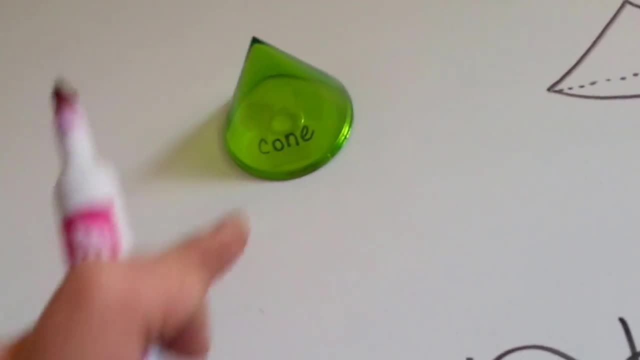 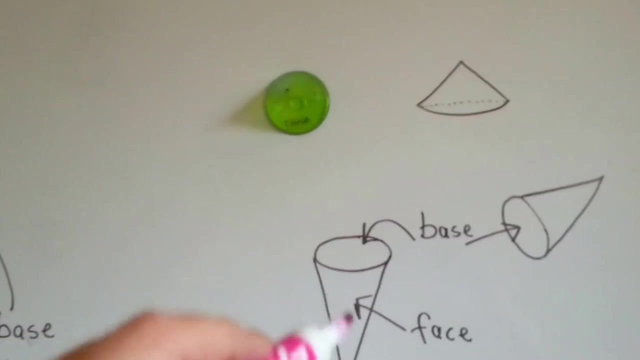 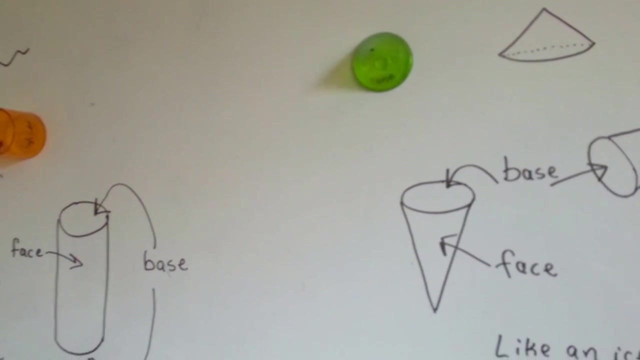 That's the cone. See how it's got a point to it. It's like an ice cream cone stuck to my board, So it doesn't matter which direction it's laying, It's still a cone And it's got only one base where this cylinder had two. 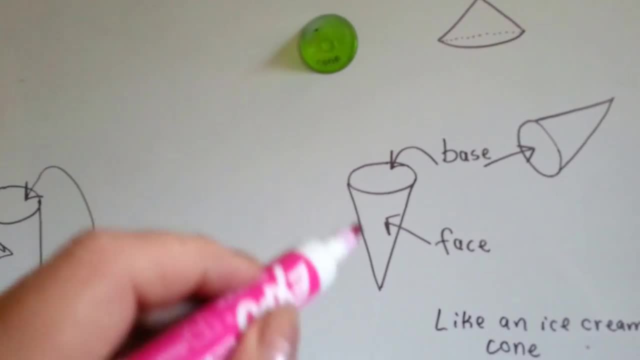 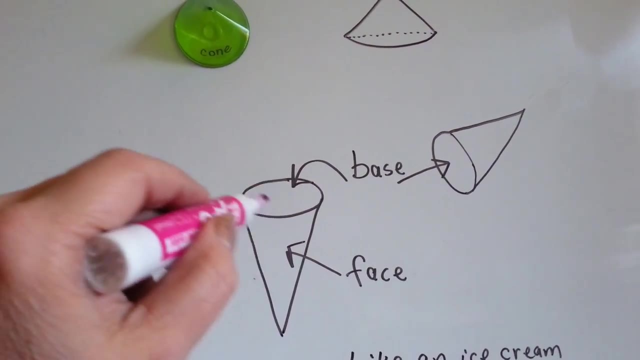 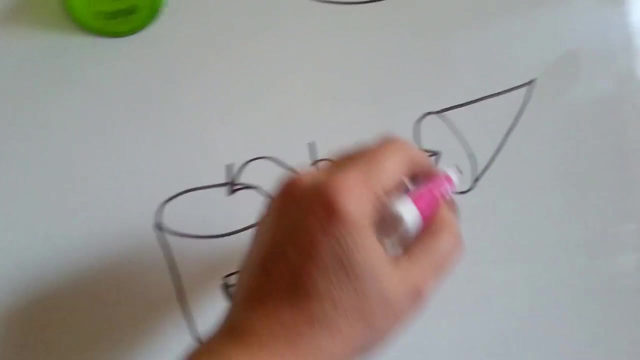 The top and the bottom. A cone only has one base, because the other end comes to a point Like an ice cream cone. So that's the face. This round flat part is called the base, And if you were to put a cut along the side here, 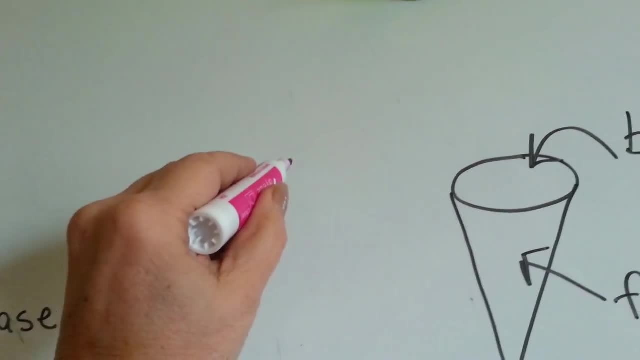 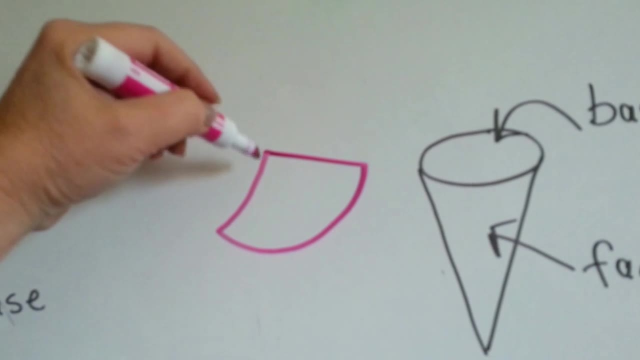 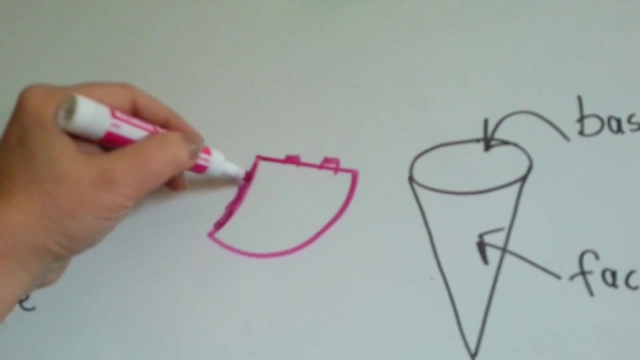 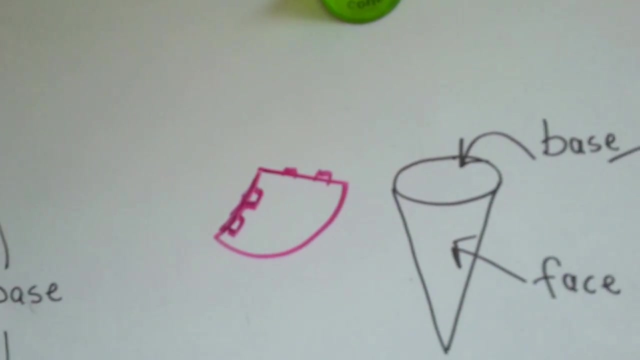 If you were to cut this open, It would be shaped like this: And then if you taped this part to this part- Let's say you had some tabs And you connected this part and wrapped it around to this part- It would end up being in the shape of a cone. 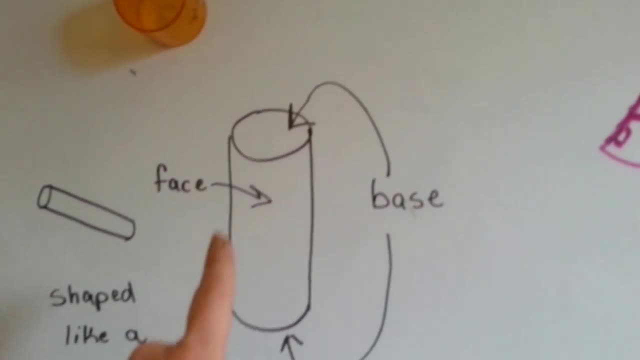 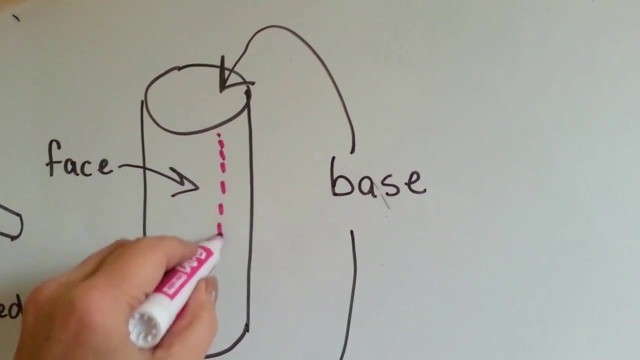 Because that's what a cone looks like opened up. Now, if you were to do that to the cylinder, It would be like the label on a vegetable can. If we just cut the label off right here And we opened it up, It would just be a rectangle. 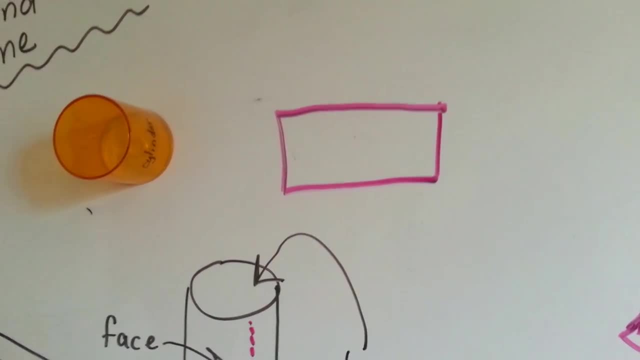 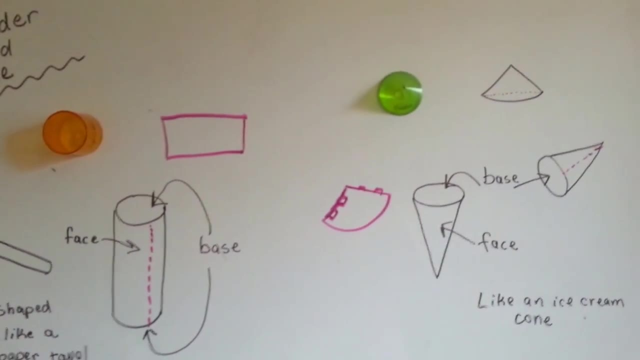 Try taking the label off of a vegetable can And see what the label looks like. It looks like a rectangle when you open it up. So that's a cylinder And that's a cone, And those are two new geometric shapes That you now know. 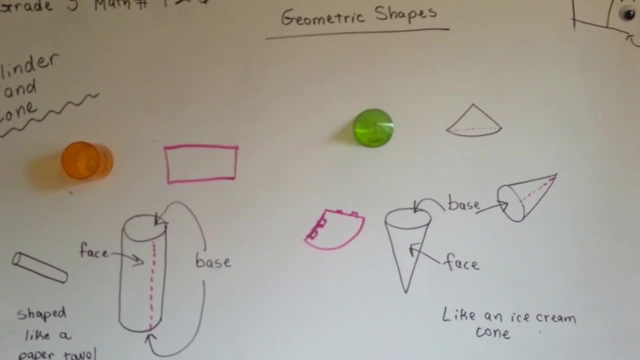 And we're going to talk about a couple more In the next couple of videos, So stay with me and see what they are. Bye.